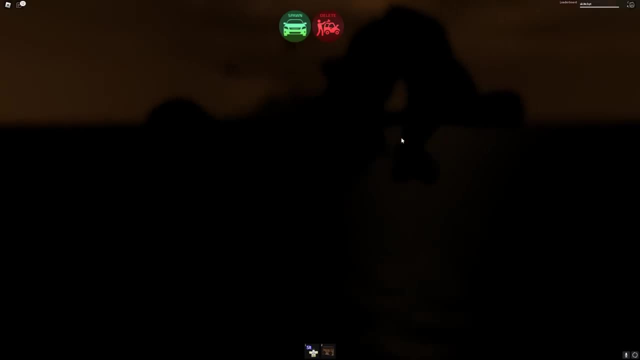 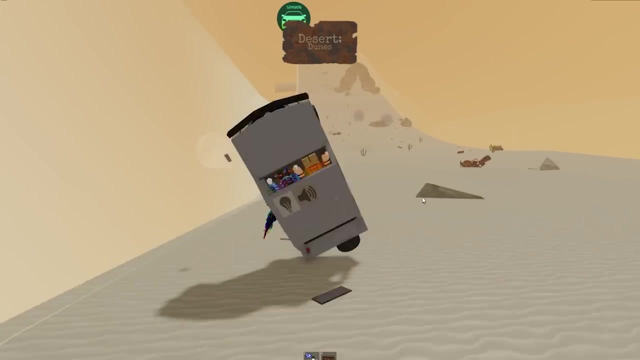 I'm dead. I'm dead. If you don't go fast enough, the snipers will get you Here. give me a ride, man. please get in. the only way I can get past the snipers- Perfect. All right, Cal, you're gonna have to bring us home, buddy. 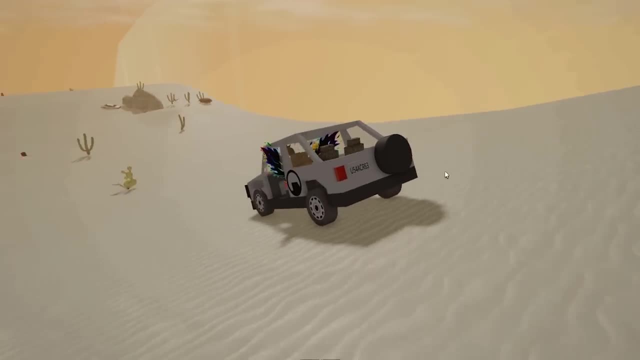 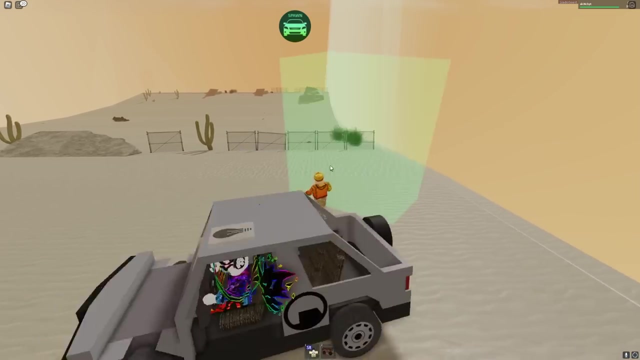 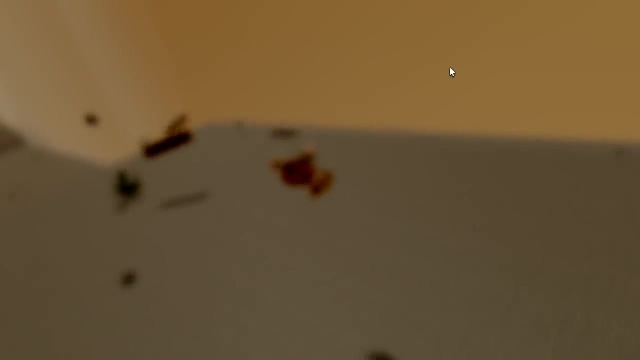 Take home country roads. West Virginia, I think you want to avoid the cactus is KAL? I don't. don't hit them on, Perp, Not we're dead. Spawn the jalopy. sorry, Cal, I'm not dying today. What did you get? a better car? I have 11,000. I get the lot. 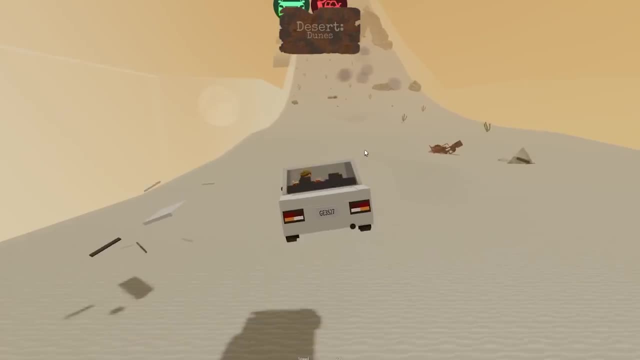 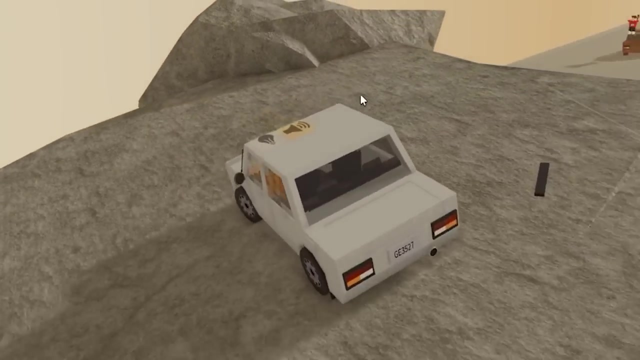 It's a lot of this- has to do slightly better then the Rustic, old, terrible car, please, no, don't die, don't die. keep going to make this jump. clean, clean, clean clean. this car is immediately already better. oh see, okay, that was a landmine. that was a landmine. 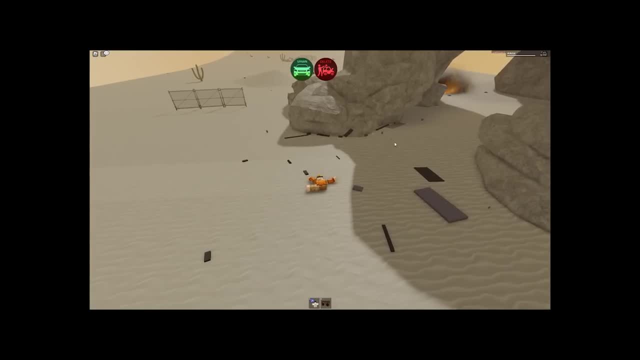 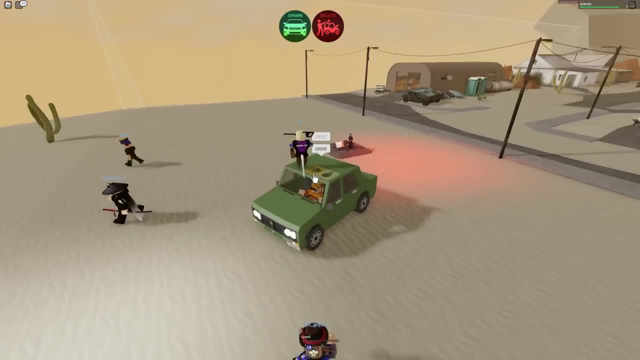 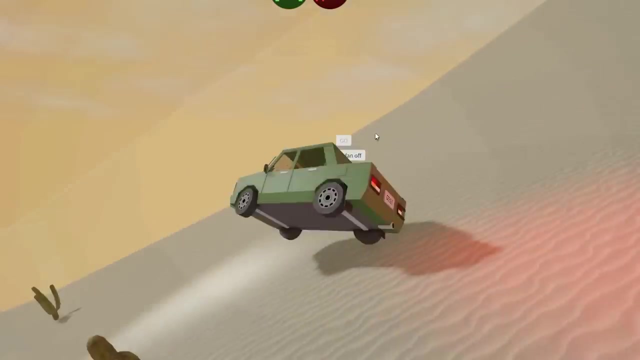 that's a lot of mines, that's so many mines. who's putting all these mines here? guys, get in, get it, get in the car. everybody in drive, drive. hey, listen, pal, i'll drive when we're full. i'm going, fine, i'm going. i'm going fine. get off my car. what is that? okay, hold on. we're okay, you are. 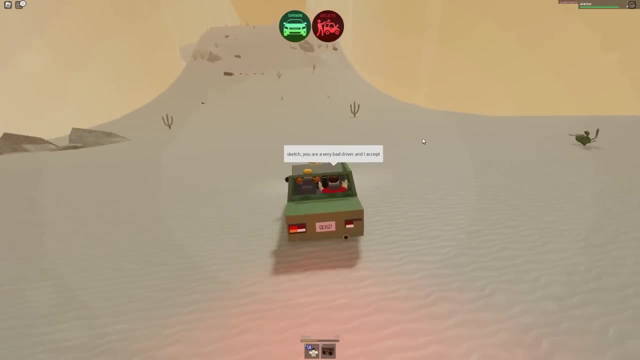 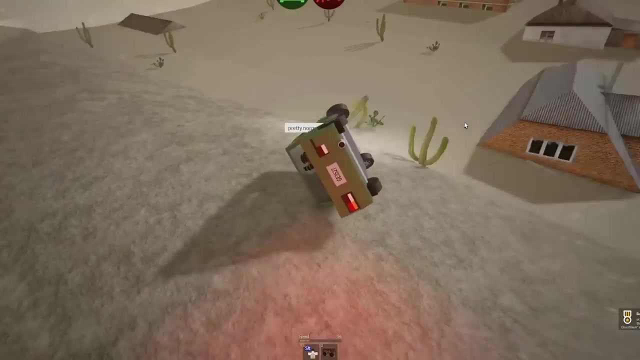 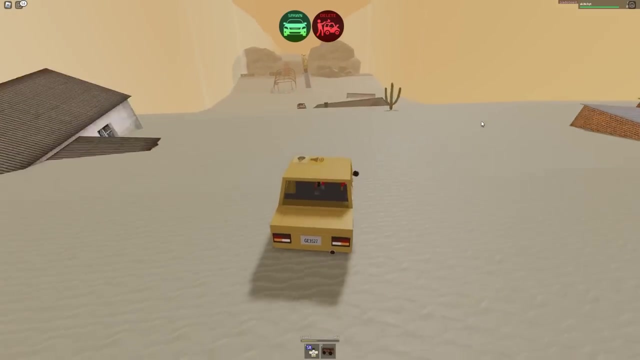 a very bad driver. don't say that to me. you kiss your mother with that mouth. i'll show you who's a good driver. buddy, please don't die. we just got, uh, the cars. i think the car is messed up. we're back, baby. i'm so scared i'm gonna run into a mine. i don't wanna blow up. we're good, we're good, we're. 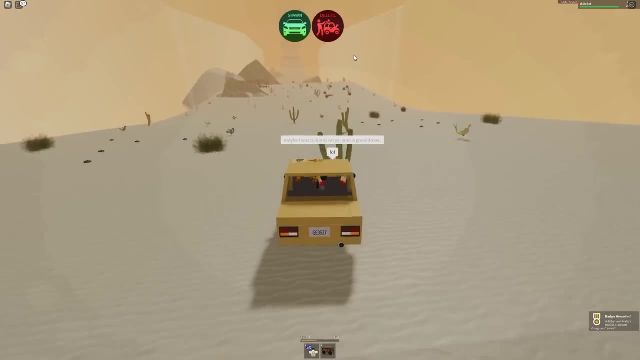 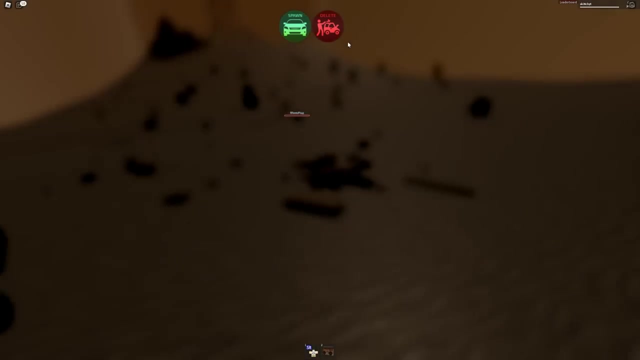 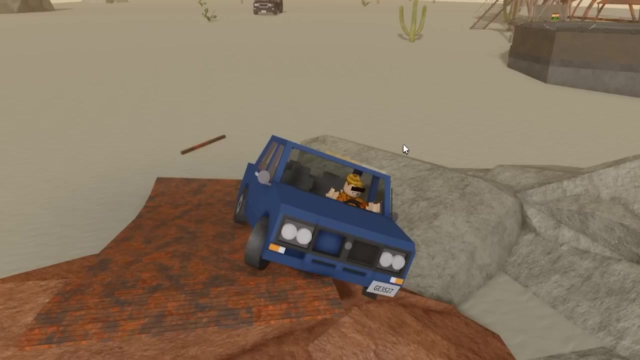 good, we made it to overgrowth, which is still the desert. there's still land mines everywhere for some reason. we don't know why. we don't know what's up with that. dang dude, this hill is huge, guys, i'm stuck. i'm sorry, don't use the ramp. don't use the ramp. 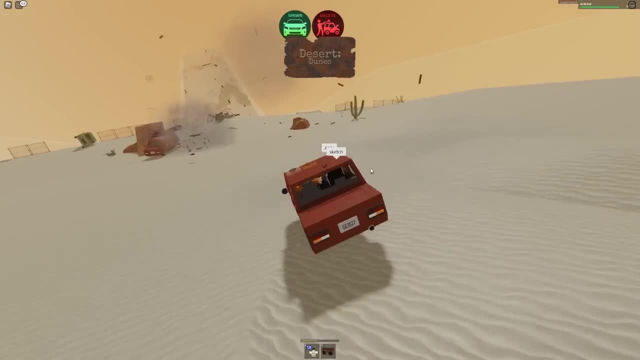 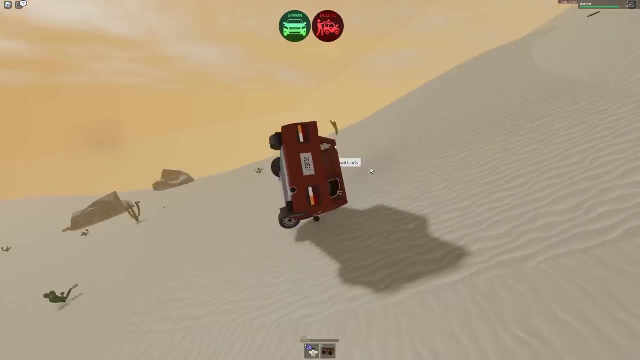 don't. i tried to warn you, man. i'm stuck here. you guys are my little captives. whoa, oh, look out, we're upside down. it's okay, i can fix this. i'm a professional driver. yeah, see that, get out of my way, partner. what are you doing? 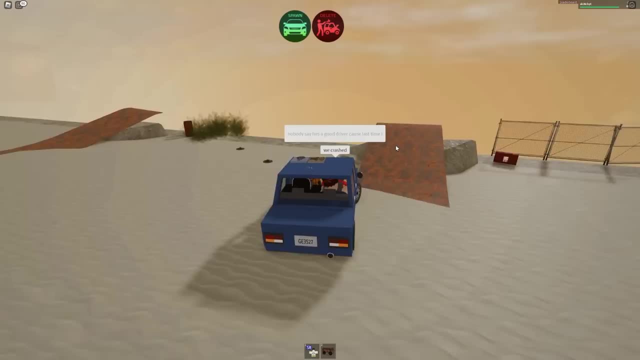 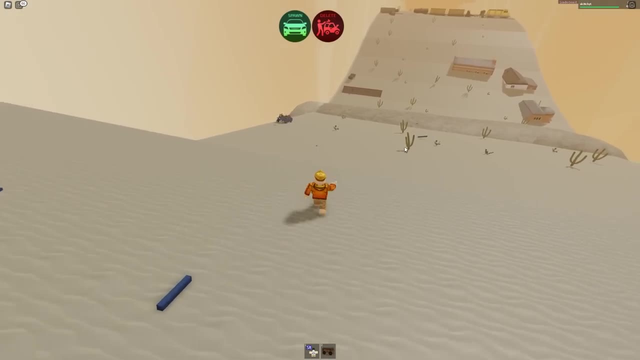 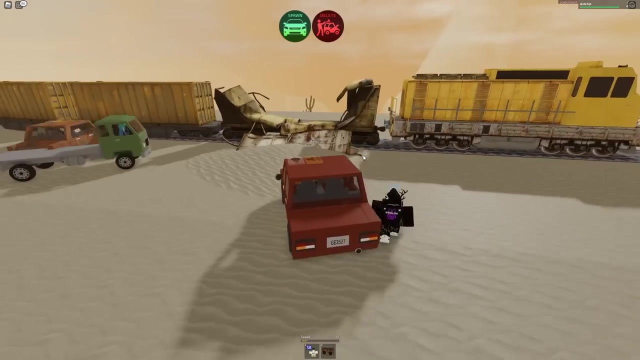 don't let us down. that was not my fault, oh my god, i'm sorry. boys, oh, oh, okay, what? how did that? how does that work? see ya, boys, sorry, got no time to spare, gotta go. oh, hold on. oh, oh my god, there we go. everybody, hold on tight, i'm not slowing down. 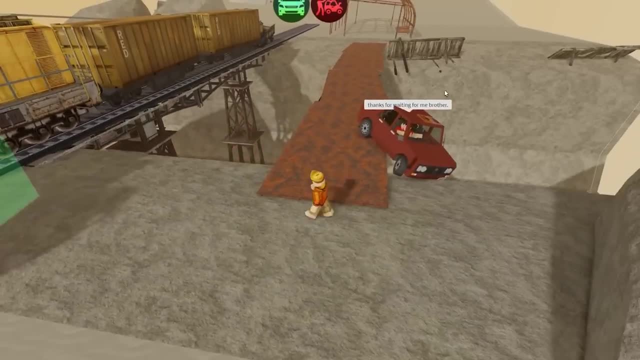 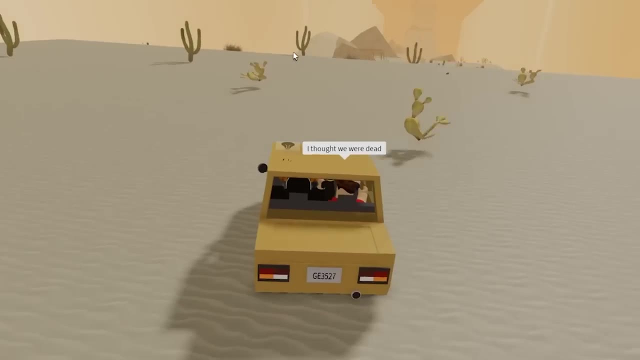 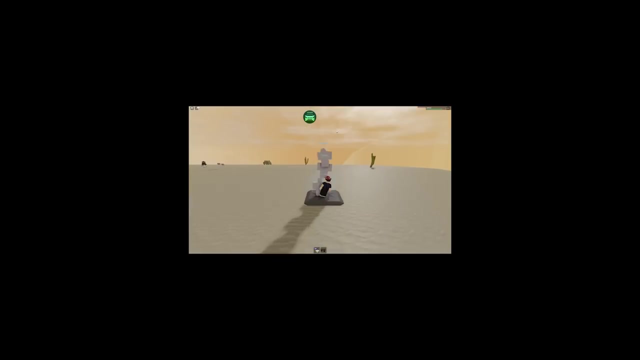 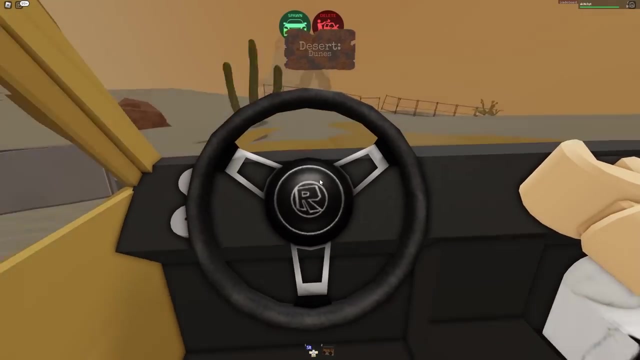 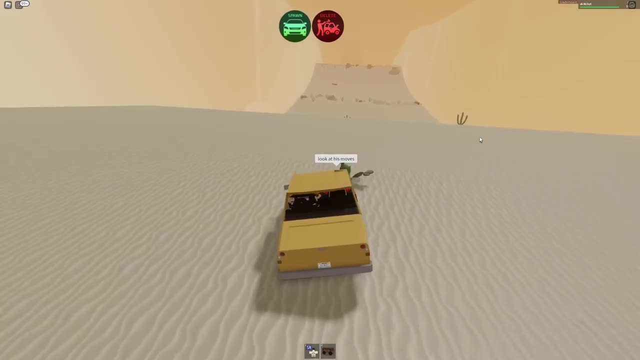 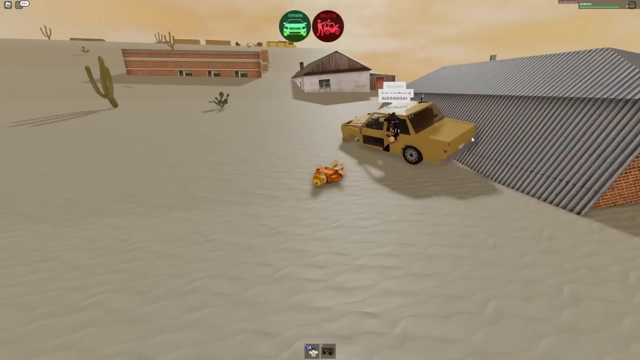 getting stuck on this bridge. whoa, We're supposed to go. We lost the tire, but we're good. Yo, Okay, Oh my God, Hold on everyone. I'm alive. Jeez, watch where you're going there, buster. 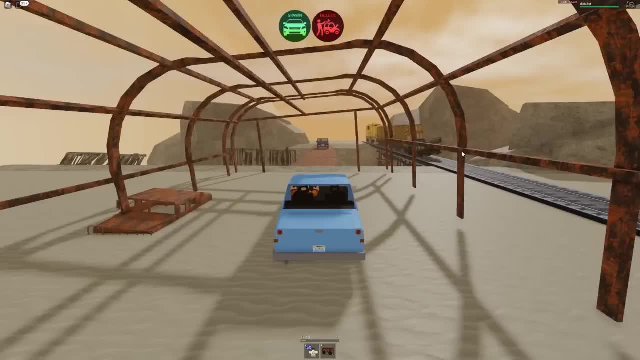 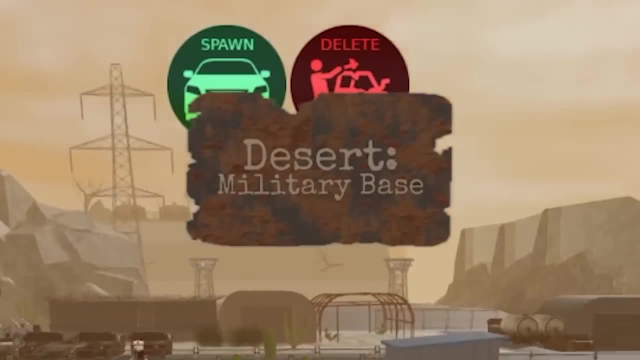 Watch it. I can't believe- I just did that- We're gonna go nice and slow over the bridge. Nice and slow? No, we're not. We're going fast. Okay, Military base, What? Okay, Oh, What, No, No. 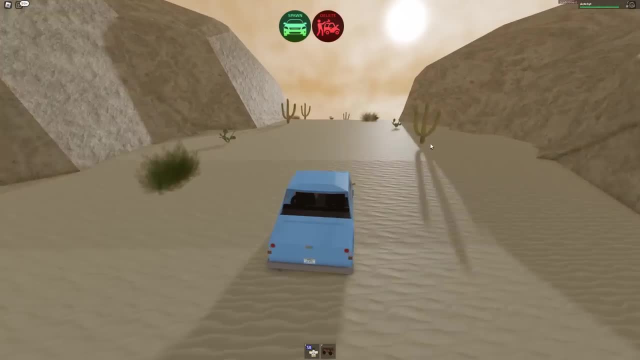 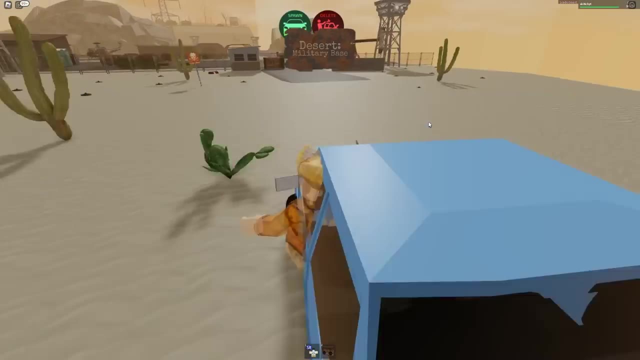 Why is there a mine right outside the military base? Military base is just up this hill. We're gonna look out for any mines. We're not going to hit the mines, We're gonna- I'm just gonna get out. I'm gonna get out. 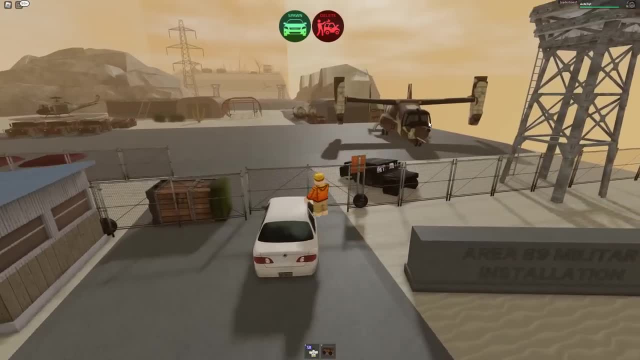 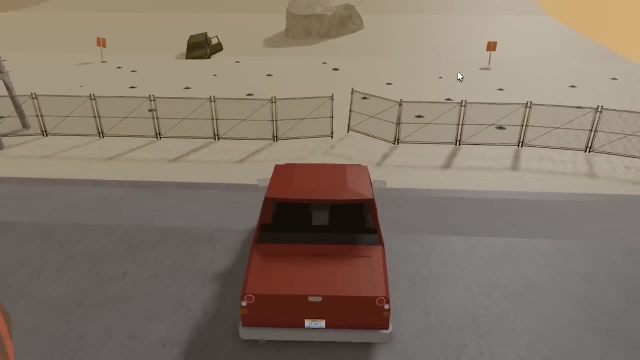 I'm just gonna walk the rest of the way. Area 89. Military installation. This is a pretty nice place. All right, let's get out of here, Please. whatever you do, no more mines. Oh, there's so many more mines right here. 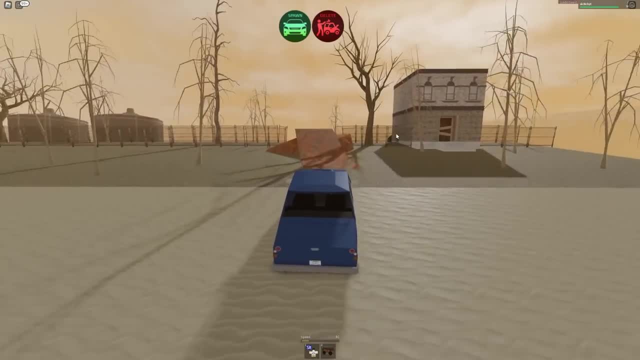 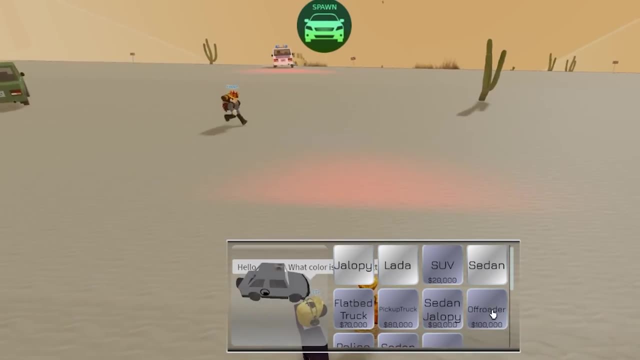 I'm getting out, I'm not risking it, I've come too far. Hey, we're going, Hey, we're moving, And we did it. A different hill Man, I cannot even- What, What? This guy's a cop car. That's cool. 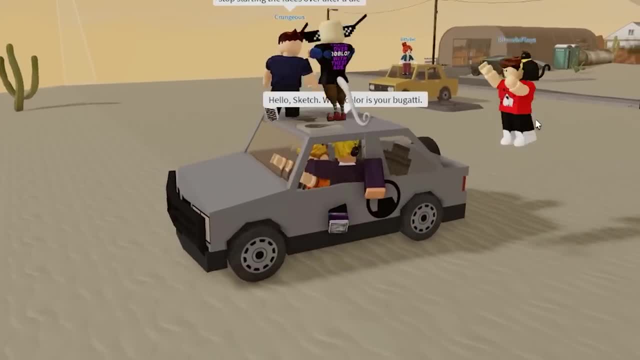 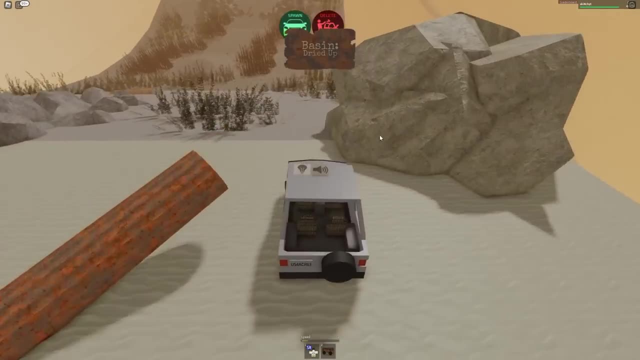 I'm gonna get the off-roader. I think, Yep, Come on, boys, We off-roading Get in This thing. better handle nice. Okay, we're back to this weird area. I don't even know what I'm supposed to do here. 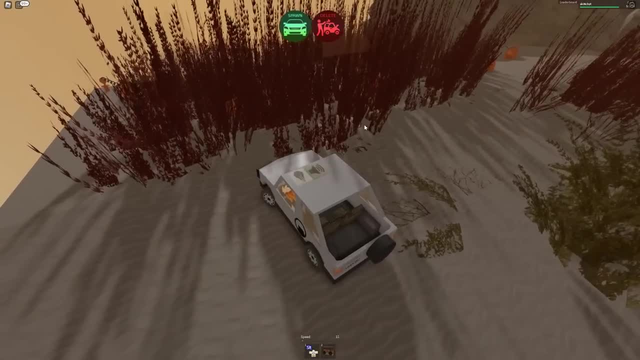 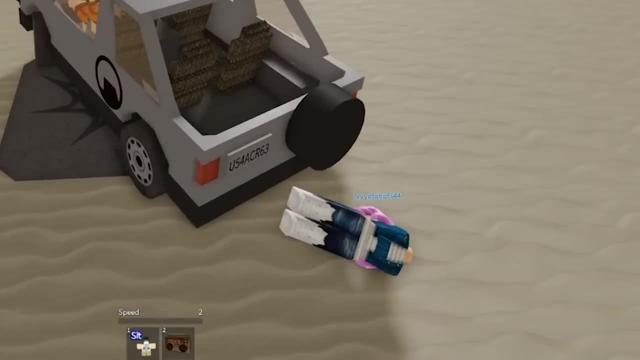 You can't even see. We're gonna creep through the grass at a safe pace. I don't know where- I don't know where to go- That explodes. What is that? Oh my God? Oh my God, I just hit somebody. 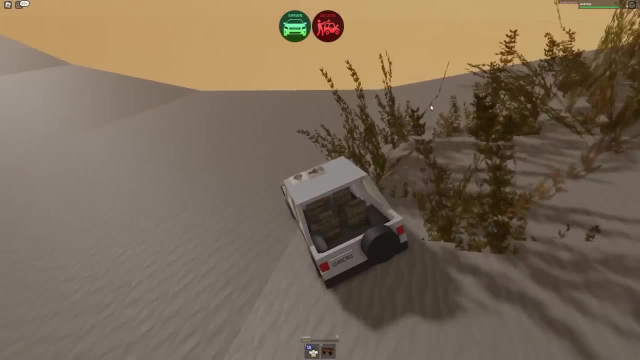 I don't even know if it's a safe idea to be in a vehicle. I feel like I would really just do the best and get the furthest if I wasn't in a car at all. I'm walking through this part. I'm not dying here. 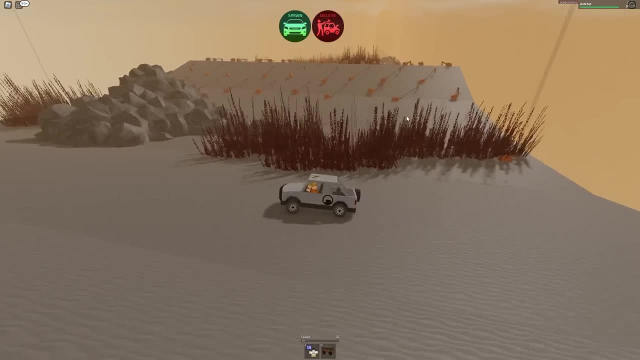 No way, Jose. Okay, we made it to the minefield. Yeah, I can see why they call it that. I'm just walking, I'm just gonna keep walking until we get past this ridiculous part. Finally, a straightaway. 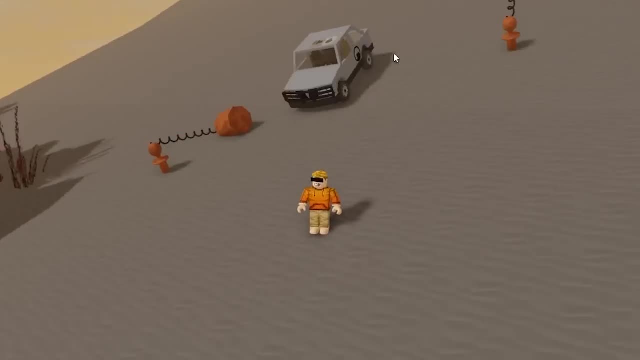 Kind of Oh, oh, oh oh, I got scared What. The car has a mind of its own. What is it doing? I'm afraid that it's gonna hide one of the things in the grass and I'm gonna hit it. 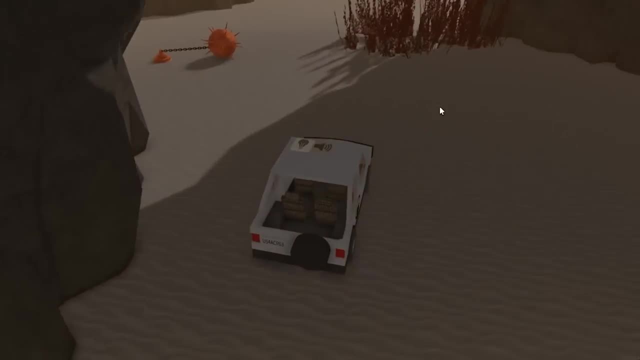 I will make it to the end of this game, Even if I have to drive it one mile, One miles per hour. The war zone? Why do they call it that? Why do they call it the war zone? Why are things exploding? 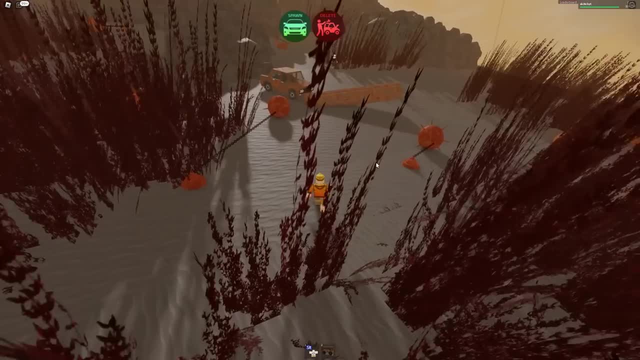 I'm so scared I'm getting out, I'm getting out of the car. What are we doing with this part on foot boys? What are you doing? You're gonna get us all killed. You're getting us all- Why? 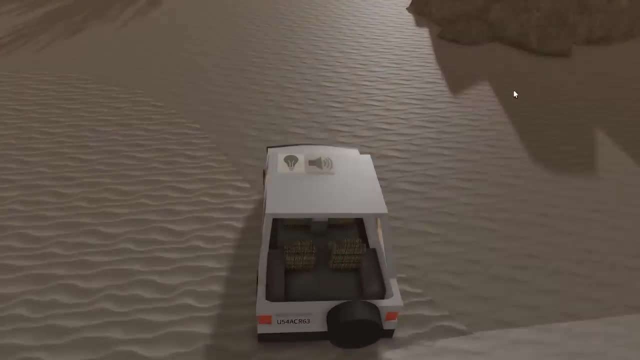 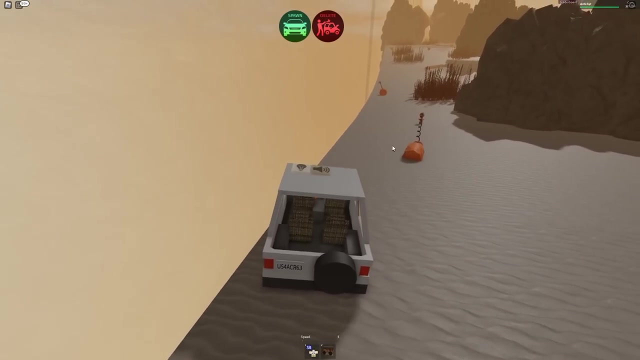 I am not going to get close to anyone. Nobody is allowed to get near me. If you come even close to me, I will not hesitate to kill you. Okay, we're just gonna squeeze by this and not touch it. We're not gonna touch it. 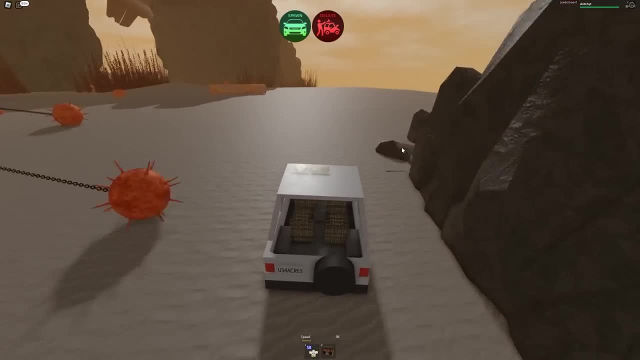 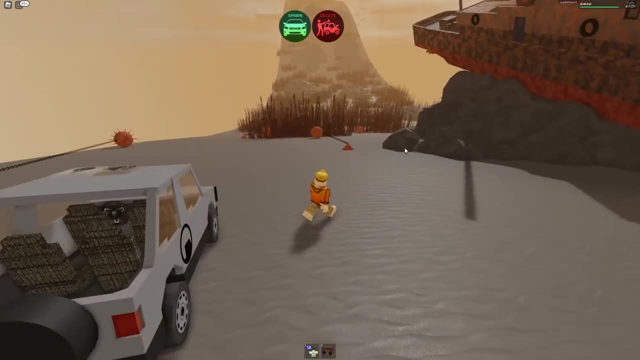 We're doing good. We're doing very good. There's no one around that could possibly ruin this for us. We're doing great, Fantastic. Now this is the part I died at. I think I'm gonna go back to the walking strategy. 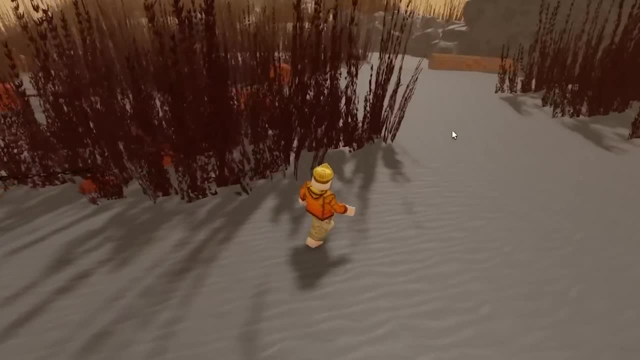 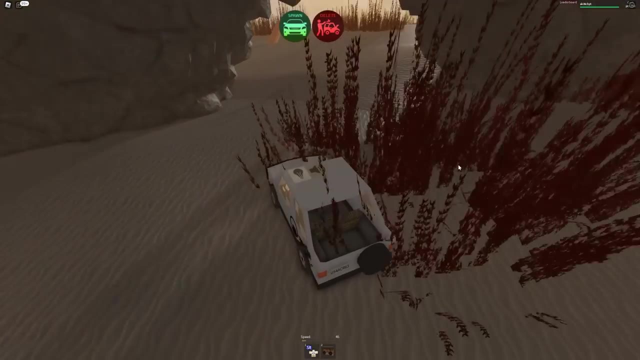 It's probably for the best. As long as we don't set off any chain reactions, we will be completely fine. How are you supposed to drive through this? This just isn't possible. So uphill is gonna be a little difficult, but I think we can do it. 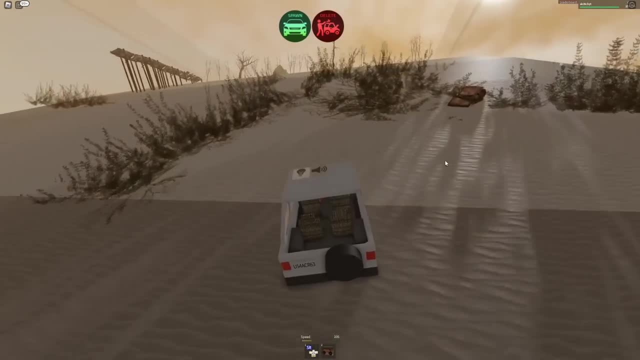 Surfacing. We're almost to the top, The tippity top of the hill. Oh, I can taste it, I can taste victory. Oh my god, we did it, We did it, We did it. We got to the unfinished part of the map. 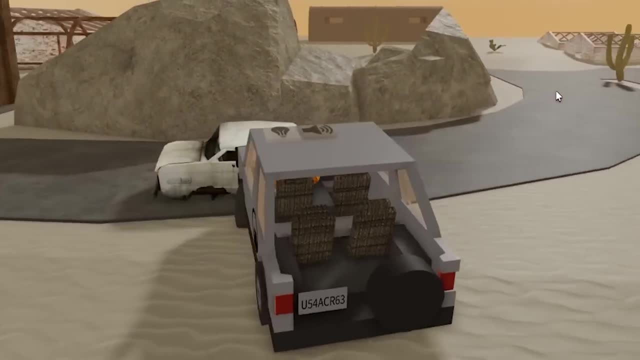 The developer didn't even get this far. He's like dang. I really made that last part impossible. How are you even here right now? I didn't even finish this part. I can't believe you left it like this, bro.